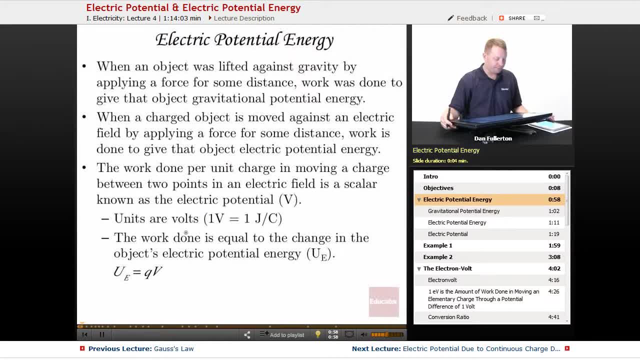 Alright, Electric potential energy. Let's start there. When an object was lifted against gravity by applying a force for some distance, we had to do work to give that object gravitational potential energy. When a charged object is moved against an electric field by applying a force for some distance, we also have to do work to give that object electric potential energy. 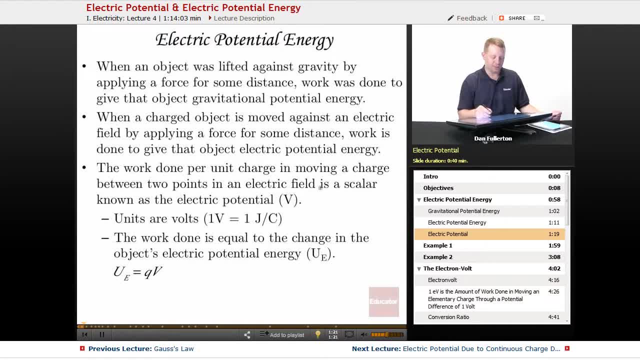 The work done per unit charge in moving a charge between two points in an electric field is a scalar known as the electric field. The work done per unit charge in moving a charge between two points in an electric field is a scalar known as the electric potential. 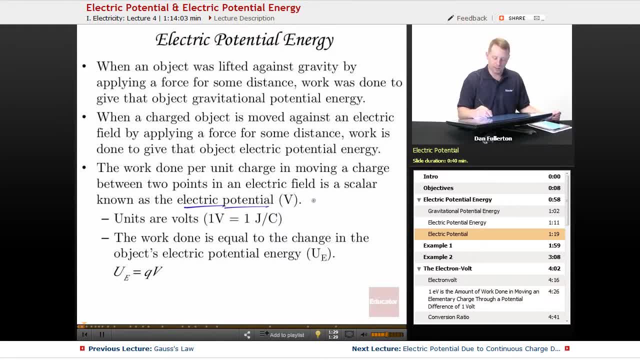 More often times you'll hear that referred to rather informally as voltage. The units are known as volts. where one volt is a joule per coulomb. The units are known as volts where one volt is a joule per coulomb. 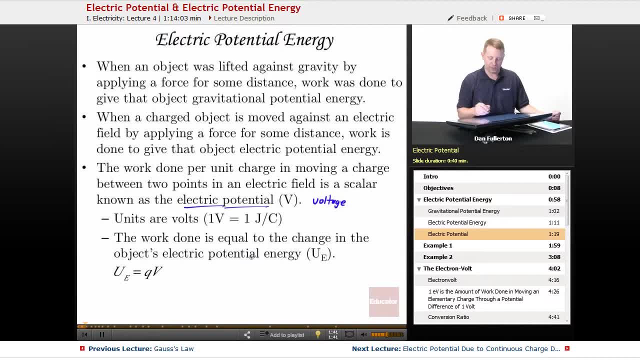 And the work done is equal to the change in the object's electric potential energy, which we're going to symbolize: capital. U for potential energy and E for electrical. where the electrical potential energy is the charge times the electric potential energy. where the electrical potential energy is the charge times the electric potential energy. 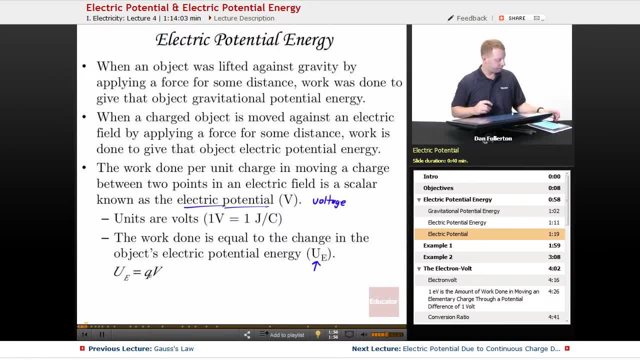 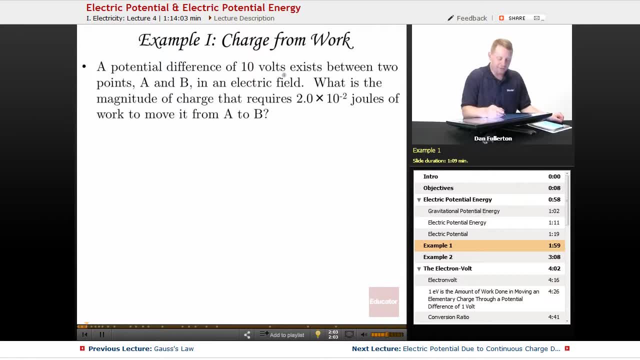 electric potential V. Alright, so taking a look at charge from work, A potential difference of 10 volts exists between two points, A and B, in an electric field. What is the magnitude of charge that requires? 2 times 10 to the minus 2 joules? 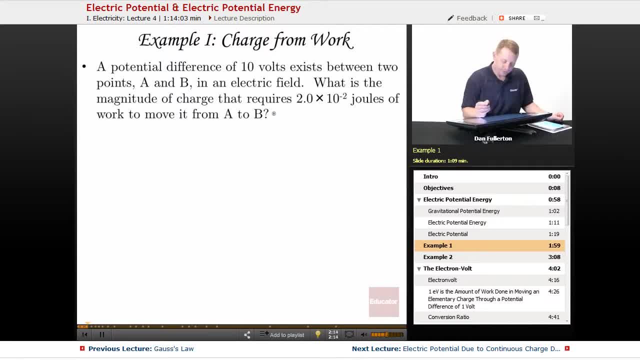 of work to move it from A to B. Well, we have a potential difference between A and B of 10 volts. We don't know charge, but we do know that the work done in moving it from A to B was 2 times 10 to the minus 2 joules. So, work going from A. 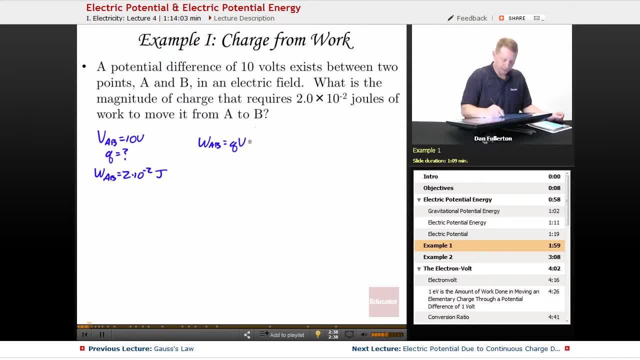 to B equals Q times electric potential. Therefore our charge Q is the work done divided by that electric potential, which is 2 times 10 to the minus 2 joules. divided by 10 volts, or charge is equal to 2 times 10 to the minus 3 coulombs. Pretty straightforward problem to start. 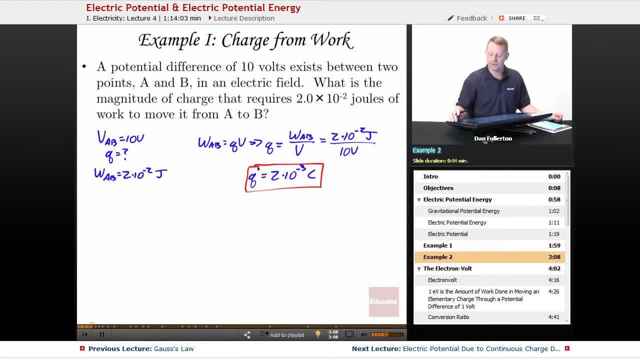 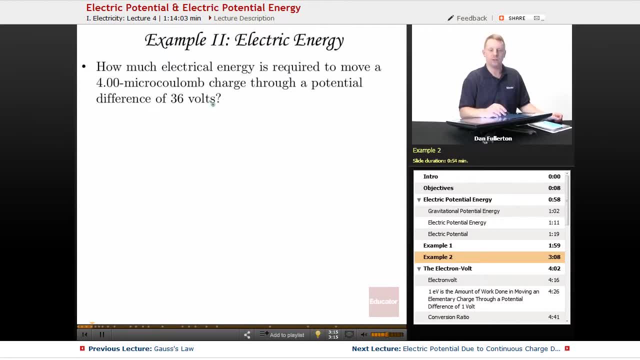 us off. Let's take a look at electric energy. How much electrical energy is required to move a 4 microcoulomb charge through a potential difference of 36 volts? Well, now we're looking for electric potential energy. We know our charge is 4. 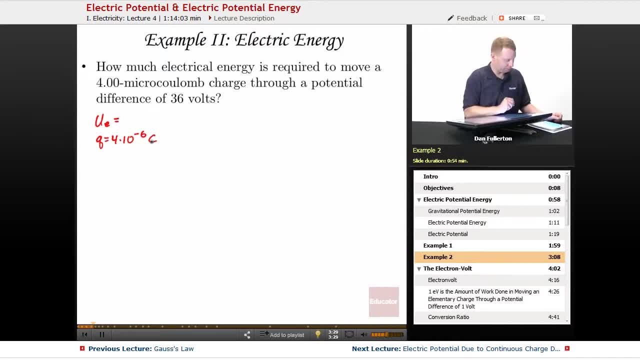 microcoulombs, Our 4 times 10 to the minus 6 coulombs, and the potential difference is 36 volts. So U equals QV, which is 4 times 10 to the minus 6 coulombs, times 36 volts, which gives us electric potential energy. 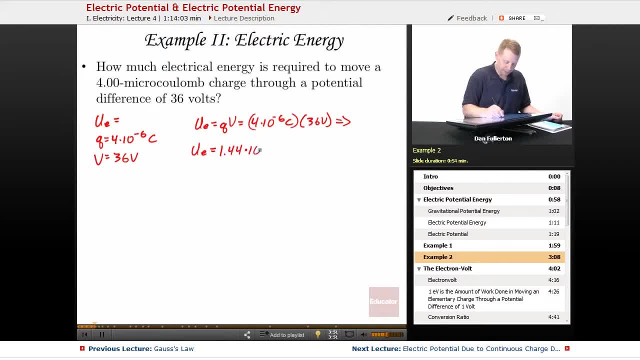 potential energy of 1.44 times 10 to the minus four Joules. Another straight forward starter sort of problem. 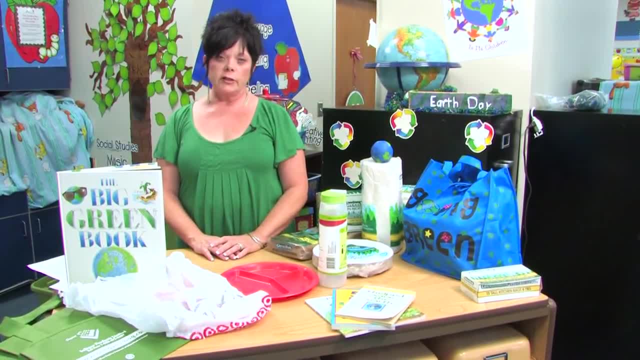 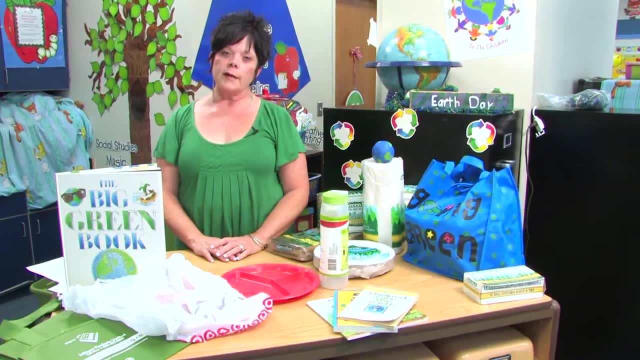 With rising energy costs and fuel costs. teaching our kids about conservation is not a choice, it's a must. Hi, I'm Debbie Noah and I'm here to help you teach your children about conservation. First of all, young children are not going to have a clue on what that 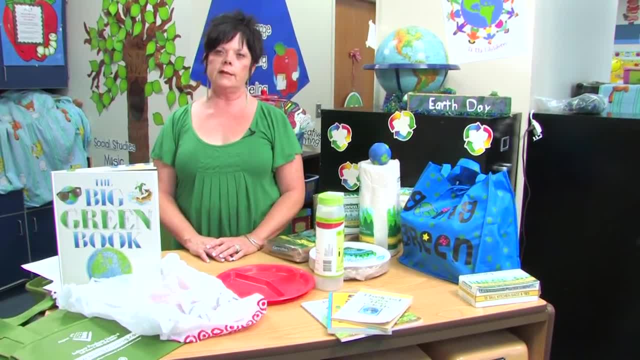 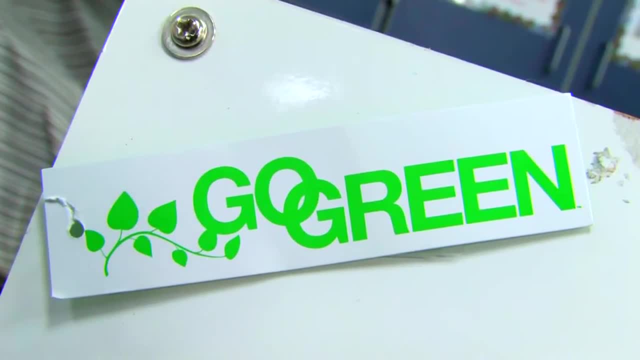 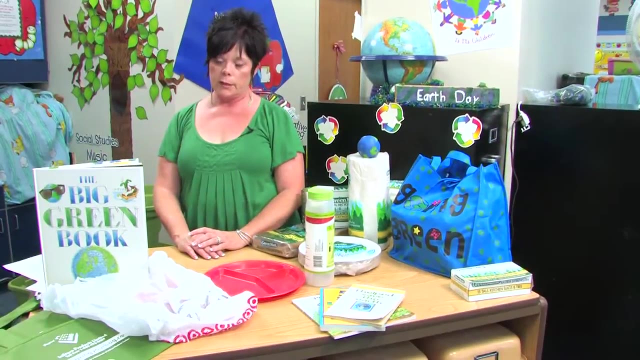 word conservation means. So you need to talk about conserving things, being practical, not wasting things, keeping things in order. But conservation goes beyond not wasting things. It's the preservation and protection of natural environments and natural resources. So conserving. 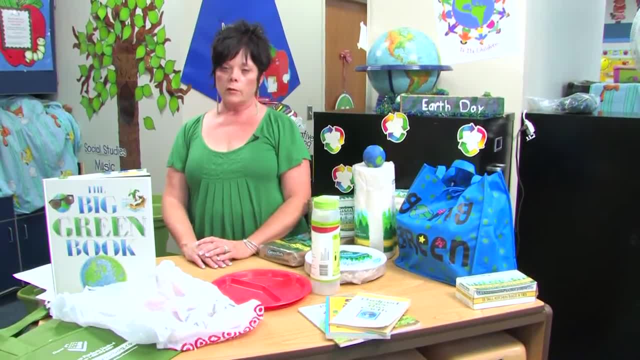 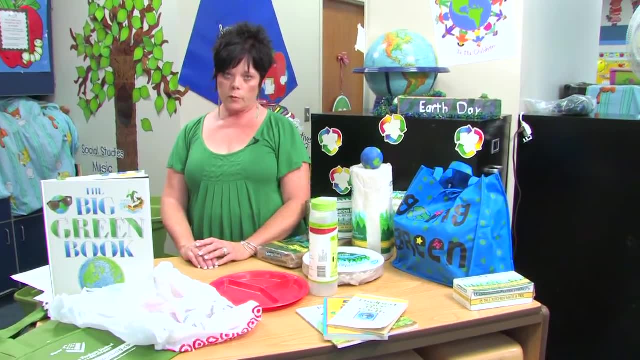 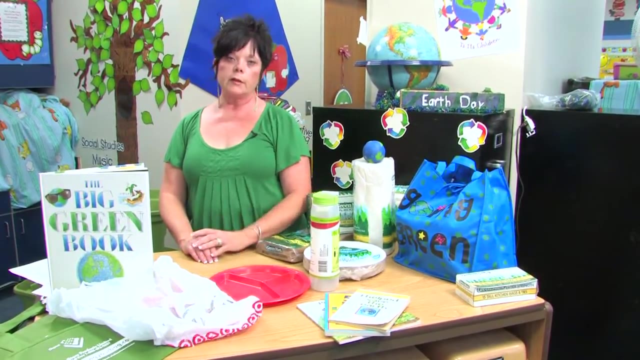 fuel, conserving oil, conserving coal- that's an important one. conserving our plants and animals on our earth is very important, Conserving air and water and soil- Things like keeping them pure and clean. How do we do that? There are lots of ways that young children can do. 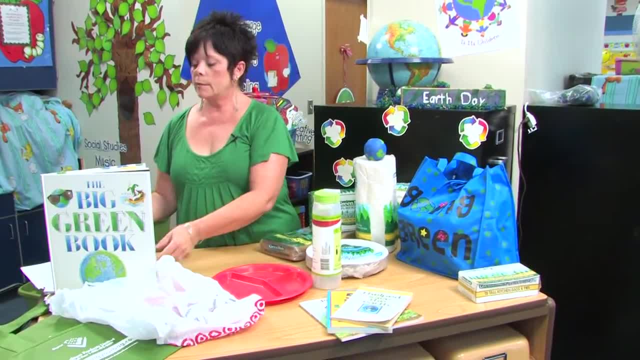 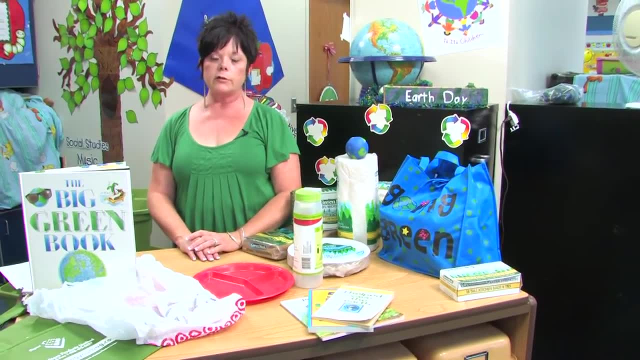 that them to conserve water. teaching them to take a shower instead of bath saves a ton of water. Not running the dishwasher unless it's half full. put your young child in charge of that. making sure that the dishwasher is completely full, Turning your faucets off when you're.